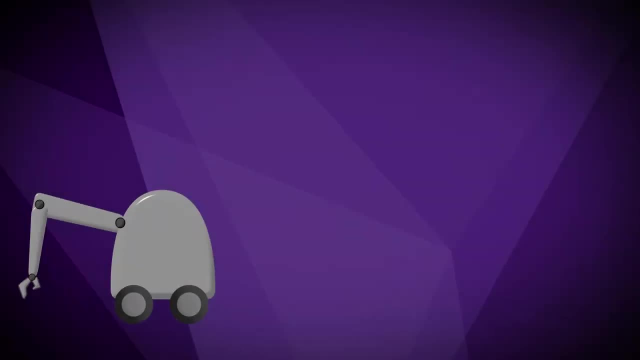 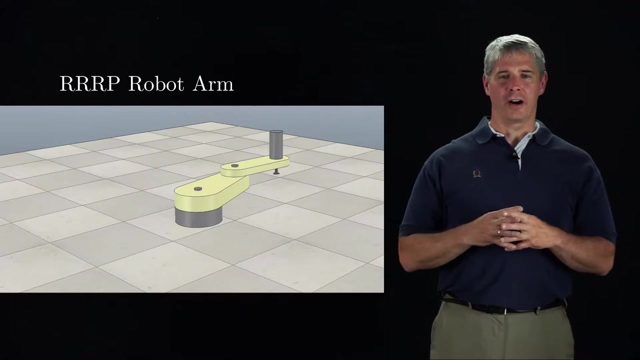 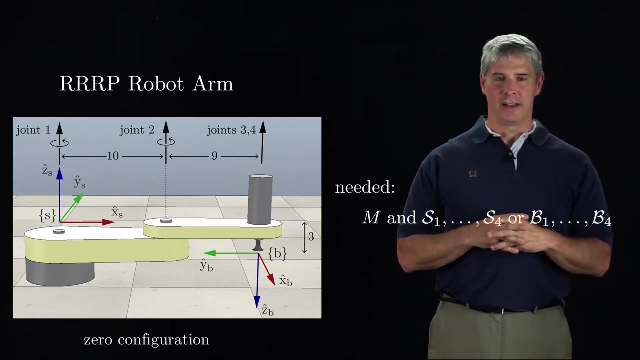 The four-joint RRRP robot, like you see here, is a popular choice for certain kinds of assembly tasks. In this picture we see it at its zero configuration. To solve the forward kinematics we need to find M, the configuration of the B-frame and the joint screw axes when the 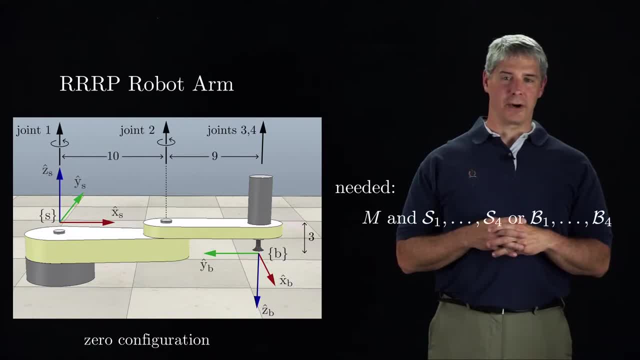 arm is at its zero configuration, Then we can use the product of exponentials formulas from the previous videos. First, let's focus on the orientation of M. From the picture we can see that the B-frame x-axis is aligned with the minus y-axis of the S-frame, The 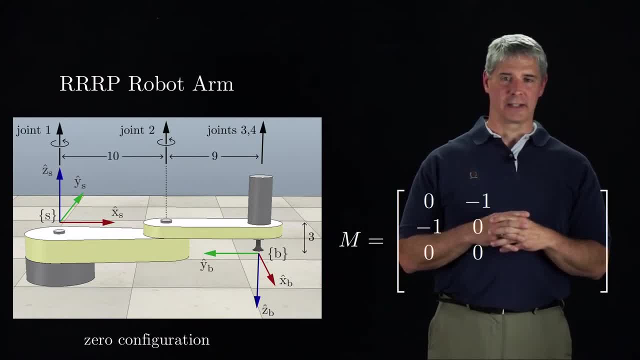 B-frame y-axis is aligned with the minus x-axis of the S-frame And the B-frame z-axis is aligned with the minus z-axis of the S-frame. Also, we can see that the B-frame is offset from the S-frame by 19 units in the x-direction and minus 3 units in the z-direction of the. 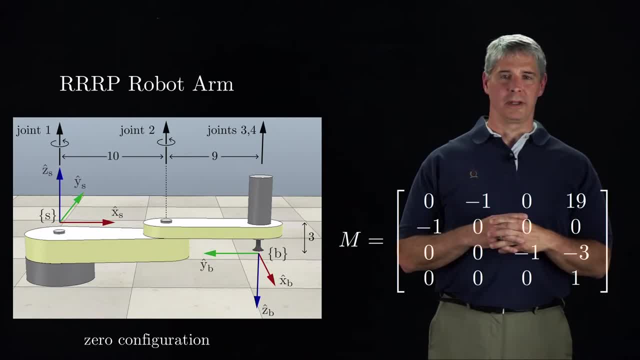 S-frame We add the row of zeros and a 1 to complete the M matrix. Next let's find the screw axis of joint 1, expressed in the S-frame. The axis of rotation is aligned with the S-frame z-axis, so the angular component of S1 is A rotation about. 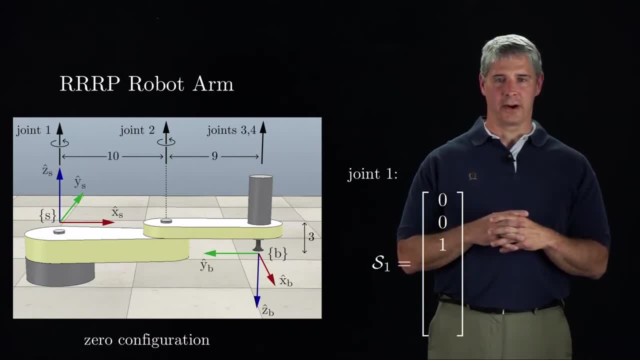 this axis causes no linear motion of a point at the origin of the S-frame, so the linear component of the screw x-axis is zero. We can also express the screw axis as B1 in the B-frame. The joint axis is in the negative. 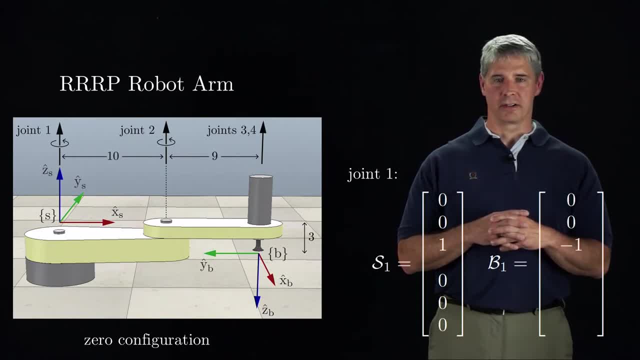 z-B direction. so the angular component is A unit. angular velocity about the joint 1 axis induces a linear velocity at a point at the origin of the B-frame. It is apparent from the figure that this linear velocity is 19 units in the minus x-B direction. 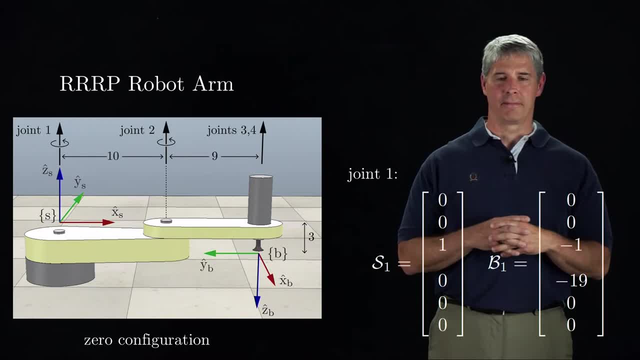 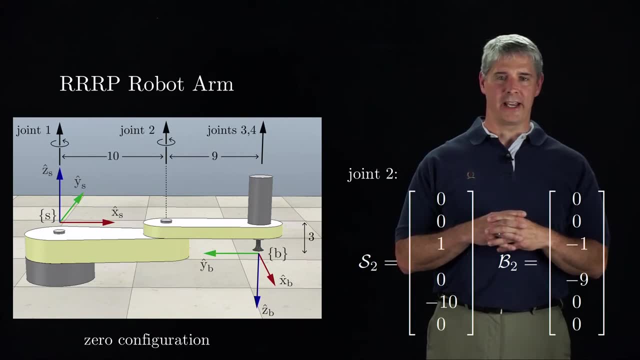 This should be readily apparent from the figure. You shouldn't have to do any math. Now let's go faster through the rest of the joints. Joint 2's axis is aligned with the S-frame z-axis, so the angular component of the S-frame 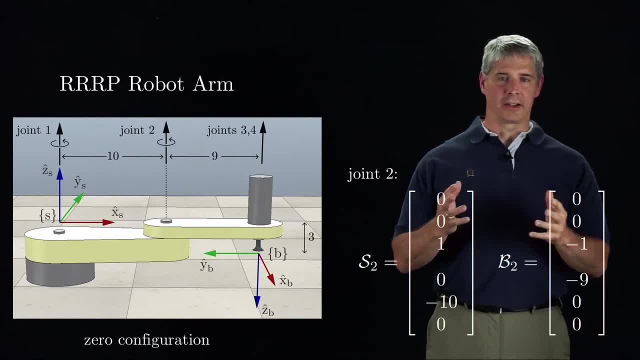 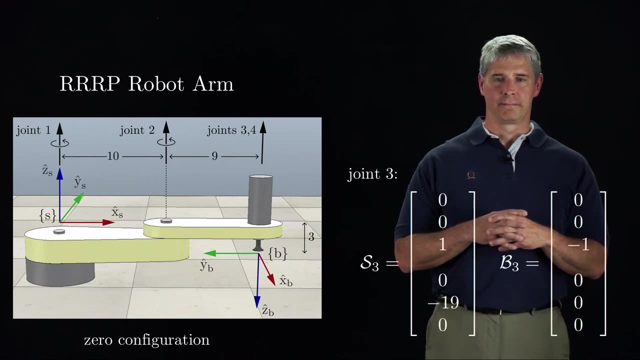 screw S2 is Unit angular velocity about. this axis induces a linear velocity at the S-frame origin of 10 units in the minus y-s direction. The screw axis B2 in the B-frame is Joint 3's rotational screw axis induces a large linear velocity at the origin of the